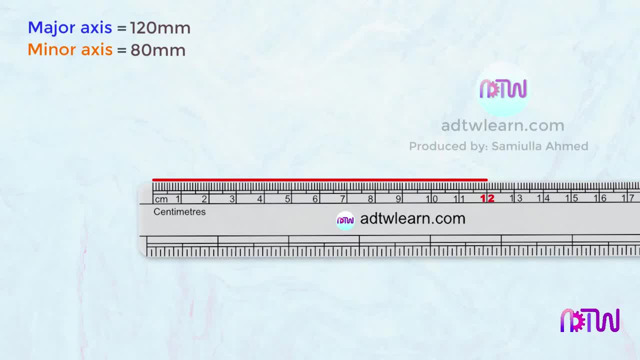 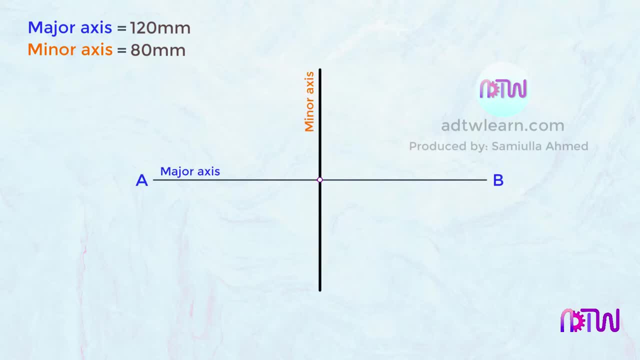 a ruler to draw a horizontal line of 120 mm in length. Name this line as A and B. After this, we need to draw the minor axis at the center of this line. To do so, divide this line into two halves. To divide, take a compass. Take the length of more than half of this. 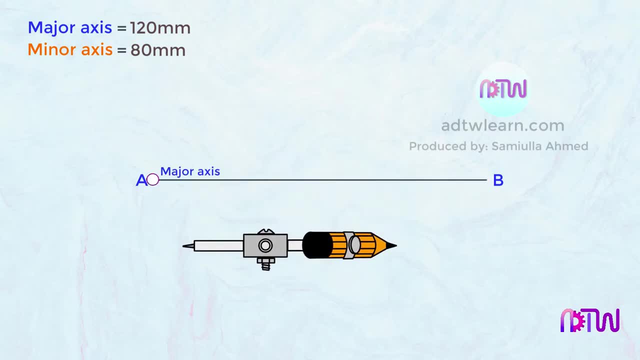 line. Keep the compass at point A and cut arcs at both the sides. Similarly, keep the compass at point B and cut arcs at both the sides. Draw a line passing through these points. This line will be exactly in the middle of this major axis. Name this intersection point as O. We can see our minor axis total length. 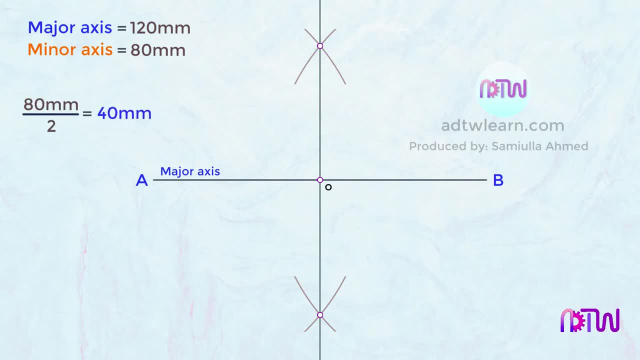 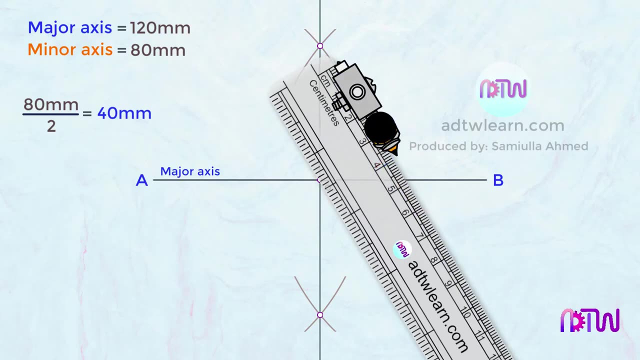 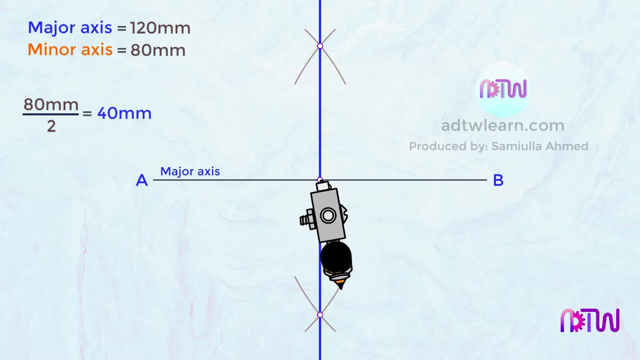 is 80 mm. Half of 80 mm will be 40 mm. Take a compass. Take 40 mm length on a compass using a scale And keep this compass at this intersection point O And cut arcs on both the sides of this line. 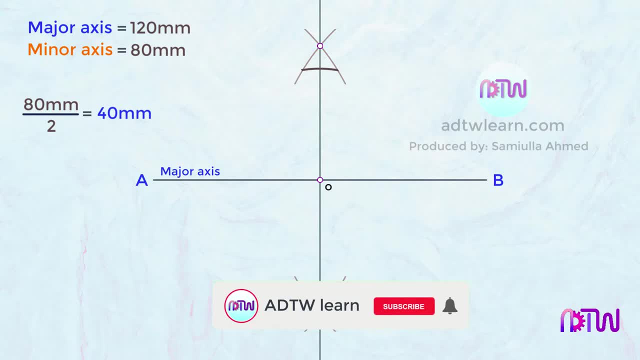 Before moving on, if you are new to ADTW, Learn, click on the subscribe button and turn on all notifications so that you can get all my latest videos as I upload. Mark these points as C and D. This length will be our minor axis. 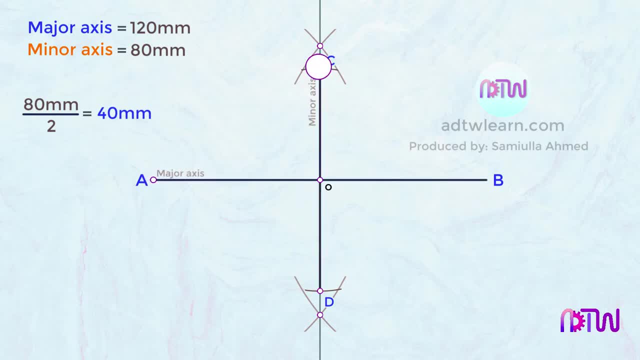 Next, we need to draw the major axis at the center of this line. To do so, take a compass at the center of this intersection, point O, and cut arcs on both the sides of this line. We will join these points A and C with a line. 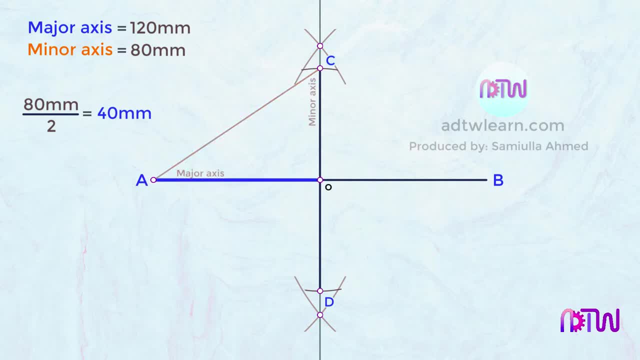 After joining. we will take a compass and take this length AO on the compass and draw an arc from point A till the minor axis line. Name this intersection point as E. Next we will take this distance between C and E on the compass and with C as the center, we will draw an arc from point E to this and 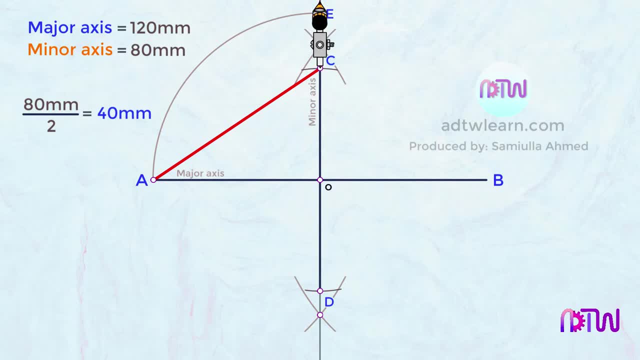 left right inclined line AC. Now we know how we will do it. We will name this point as F. After this, we need to divide this line Af into two equal parts. So to do that, we will take a compass. take some length on the compass, which is: 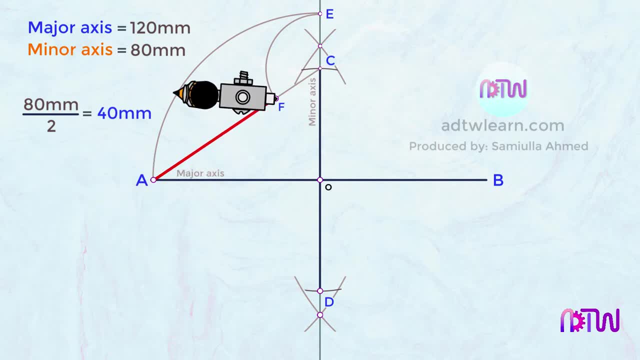 more then 1 dong the length of this line and, using F as the center, we will draw an arc on both the sides of this line. Similarly, This is theszvesquimp3 And a letztesant from point F: Using A as the center, cut arcs on both sides of this line. 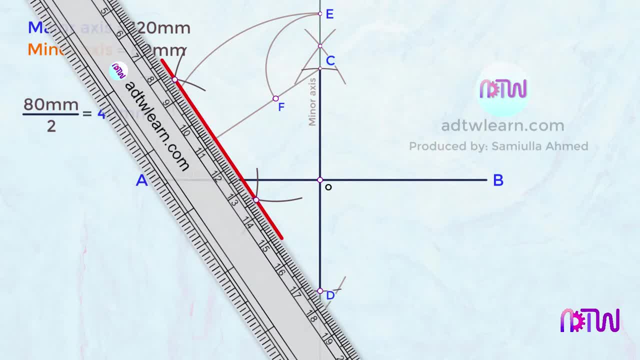 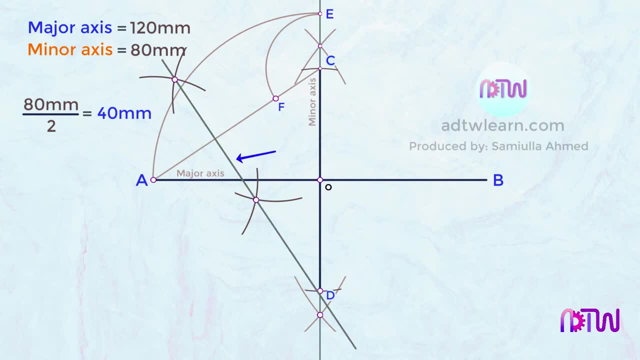 Draw a line passing through these points, See that this line is passing through the minor axis line. This line will be exactly at the center and perpendicular to line AF. This intersection point will be our point number 1, and this intersection point will 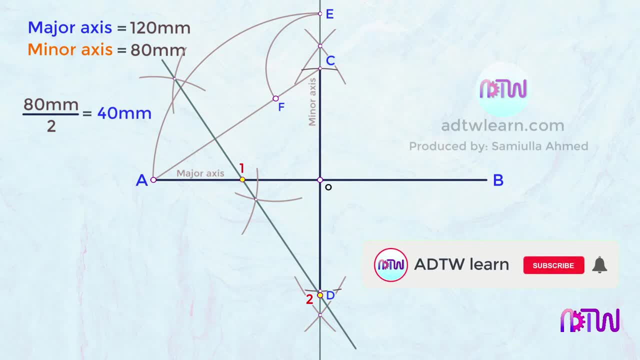 be our point number 2.. To mark the other two points, take a compass, take this length between points 0 and 1, and cut an arc on the other side of this major axis. This will be our point number 3.. 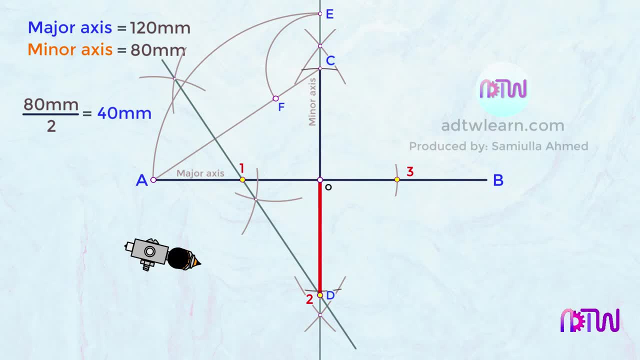 Next, take this length between points 0 and 2 on the compass and cut an arc on the other side of this line. This point will be our point number 4.. Therefore, we got all four points. After this, we need to draw a line passing from points 4 and 1, and extend this line. 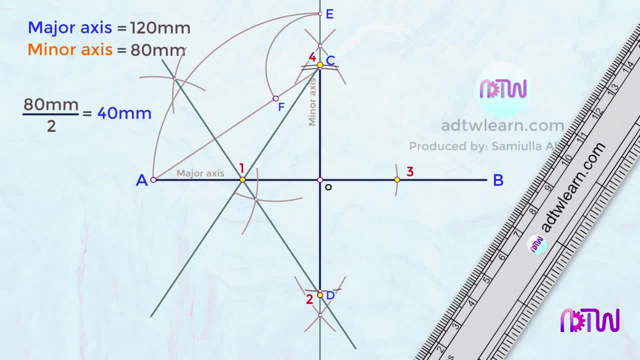 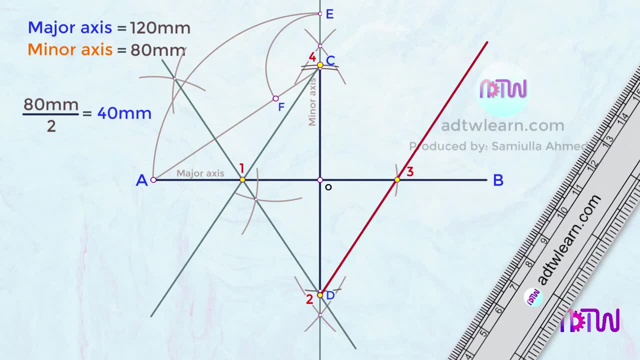 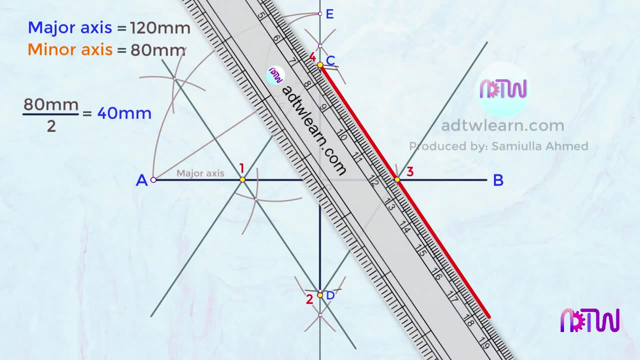 up to some length. Similarly, draw a line passing from points 2 and 3, and extend it up to some length At last. draw a line passing from points 4 and 3, and extend it up to some length. These lines will help us in getting the length of a compass. 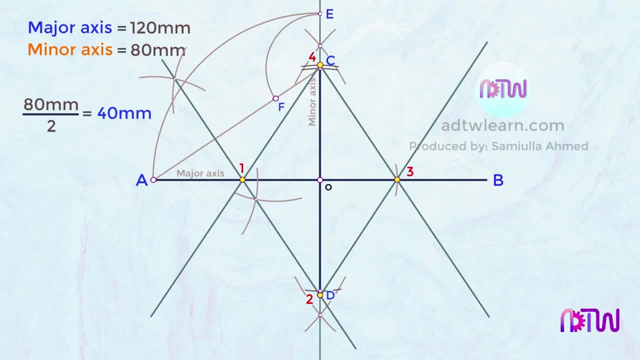 Thanks for watching. Next, we will be drawing an ellipse arcs. After this, we have to draw arcs by taking these four points as the centers. Take a compass, Take this length on the compass, Use this point as a center and draw an arc from this line to this line. 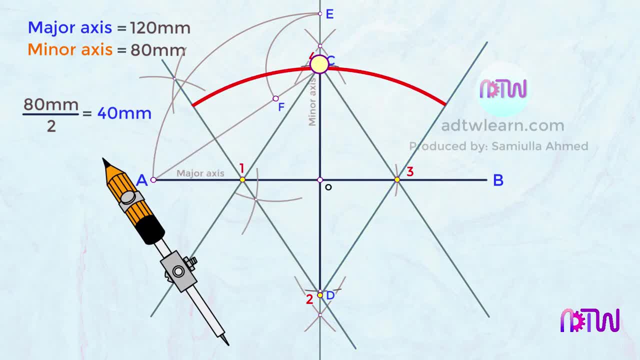 Similarly, keep the compass on point 4, and draw an arc from this line to this line. Next, we will be drawing a line passing from points 5 to 6.. Next, we will be drawing a line passing from points 6 to 6..